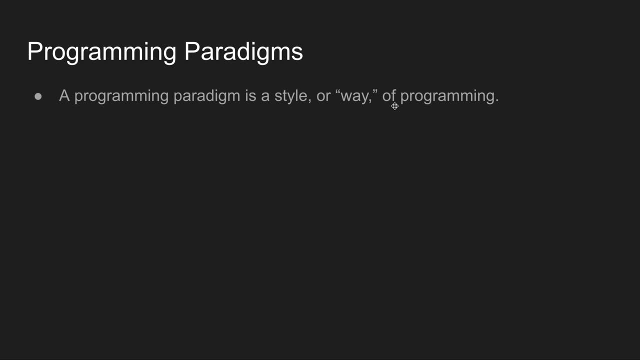 programming paradigm is a style, a way of programming. So if suppose, if we can relate this thing with the real world. For example, in India there are n number of actors in cinema field, So each actor has some unique style, So that unique style can be copied by n number of actors. 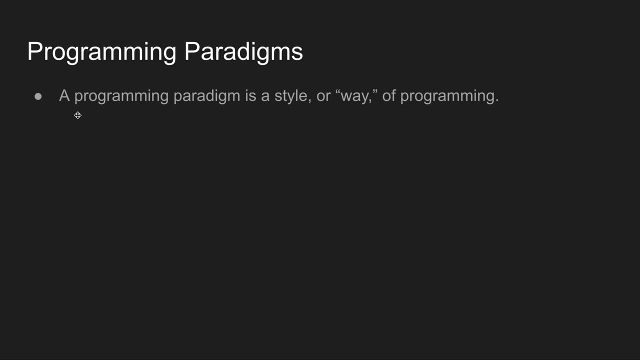 So this paradigm defines: it is a style. A programming paradigm is a style, a way of programming. So for a programming paradigm it follows some style. If some languages follows this style, then that could be fall under this bucket. So this is the common and basic definition. 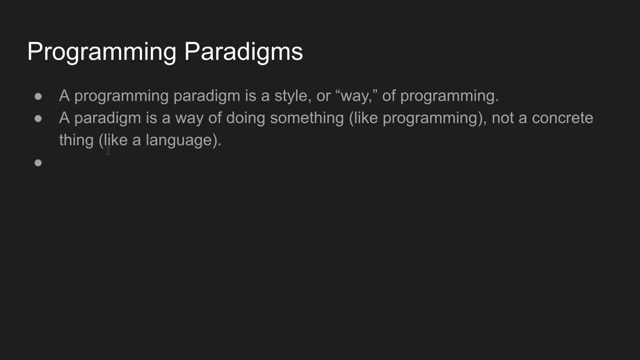 of programming paradigm. Now, the second definition is: a paradigm is a way of doing something, like programming, not a concrete thing like a language. So this is a style. it's similar to blueprint: Blueprint of doing something, but it's not a concrete thing of doing something. 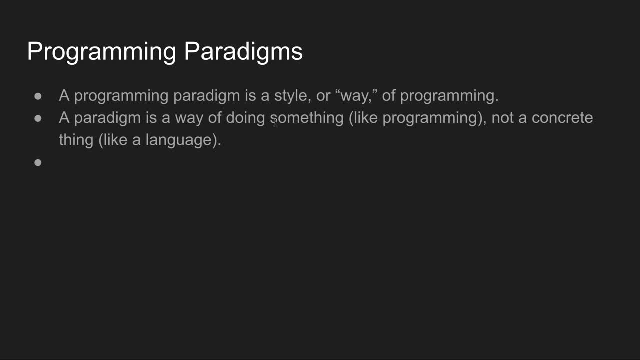 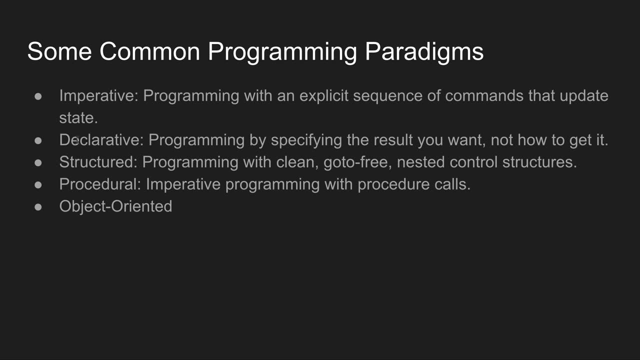 This is just a blueprint. Any languages that follows this blueprint will fall under this bucket. So there are n number of programming paradigms. So imperative declarative are the most used programming paradigms in 1950s and 1960s. 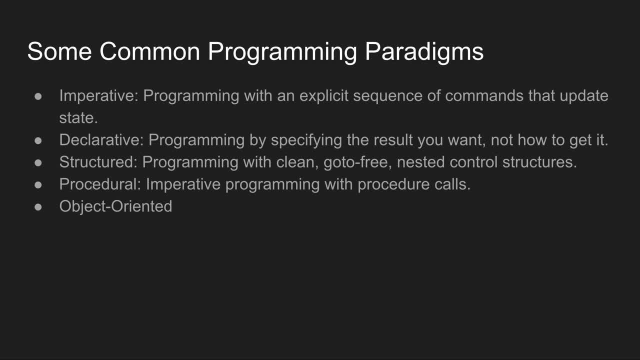 And then structured and procedural came into existence, and then object oriented programming paradigm. Nowadays, object oriented programming paradigm is playing a major role in most of the programming languages. For example, java is one of the mostly used programming language which falls in the object oriented programming language. In this course we will try to focus more about. 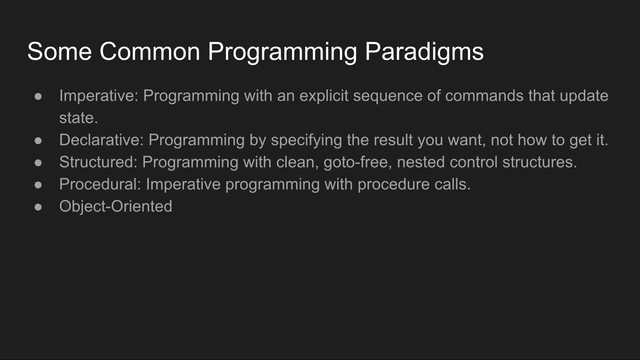 object oriented programming languages. We will try to cover each concept and we will try to analyze the importance or context of object oriented programming And we will try to see the uses. we will try to relate the object oriented programming concepts with the real world and real life examples. So we will try to cover everything. We will try to cover. 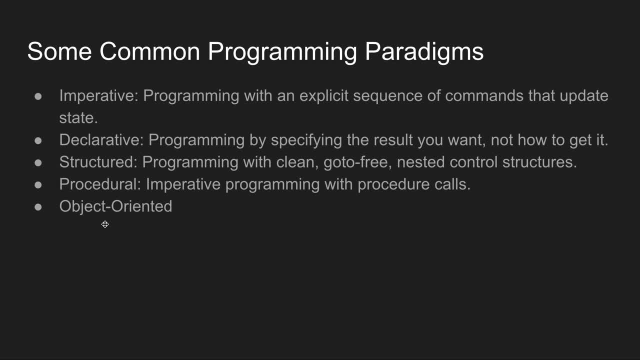 each and everything about object oriented programming paradigm in this course. So we will try to cover imperative, declarative, structured, procedural in a brief manner. So our main focus would be on object oriented programming paradigm. So first, what is imperative: This is the one of the oldest style of programming paradigm.